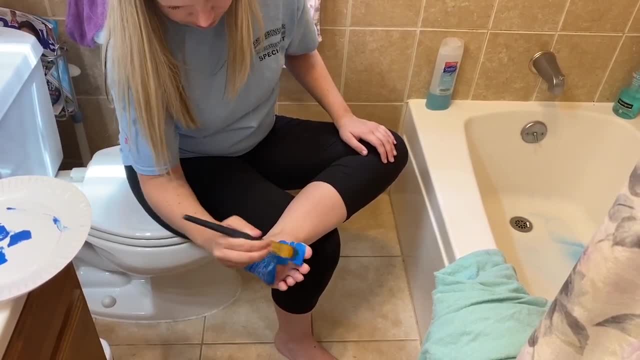 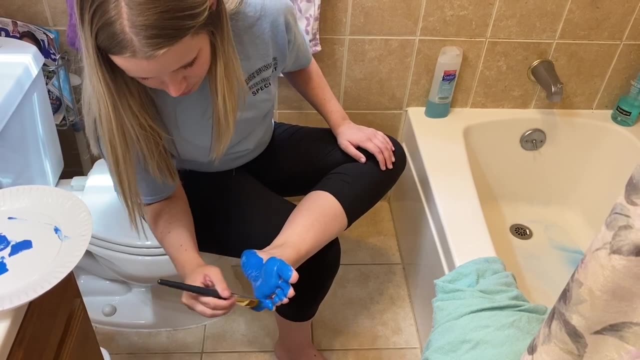 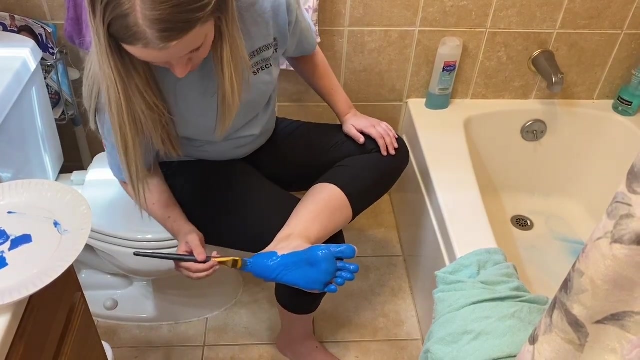 Nice and thick. It may tickle a little bit, That's okay. If someone at home could help. if you are a little confused or if you need some help getting all the pieces of your foot, somebody at home can help. That can be a great first step. 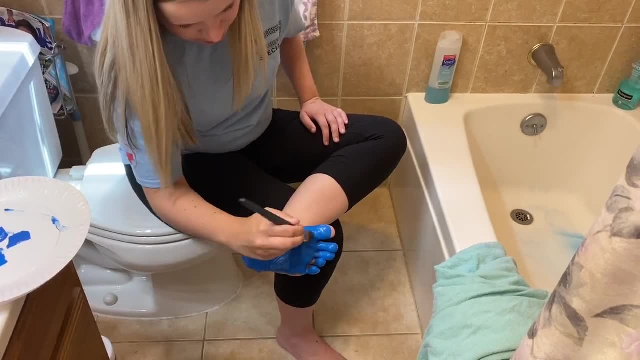 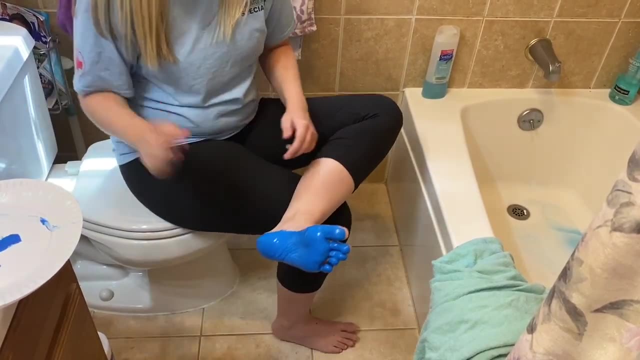 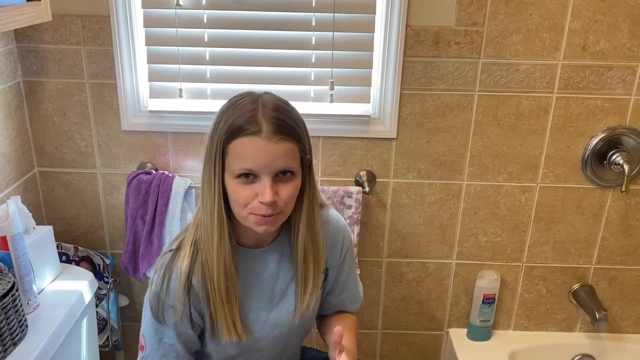 If you want to go in a second coat, that's fine too. The better the paint, the better it will stick on the paper. Okay, So my foot is completely covered in paint. It is now time to press it onto the paper to make the body of our superhero. 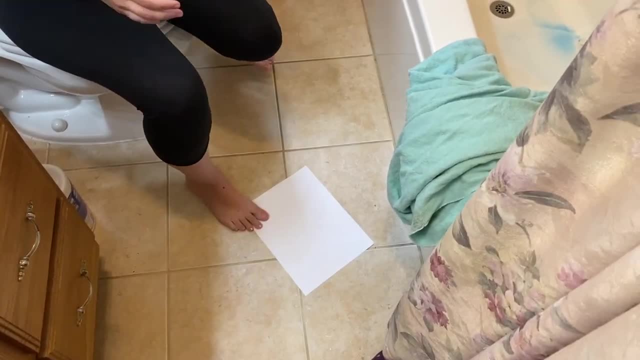 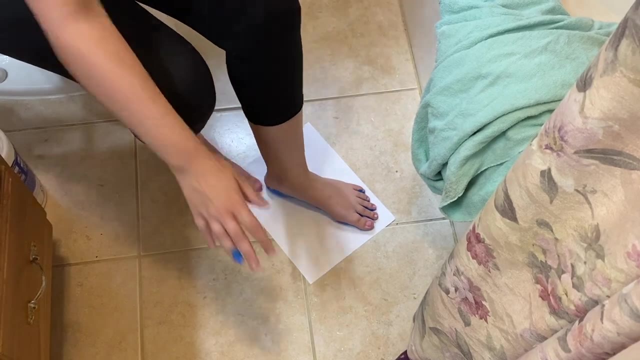 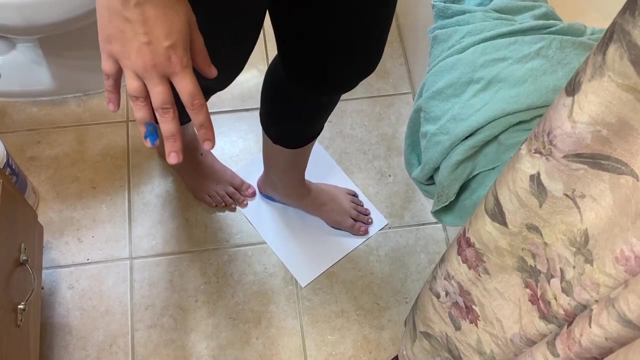 So I suggest holding it down with either a toe or if you have someone that's helping you, they can hold down the paper as well. And in the corner I'm going to press, I suggest standing up. Count to five. One, two, three, four, five. 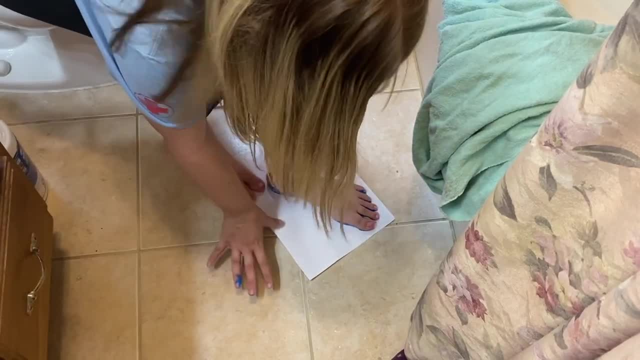 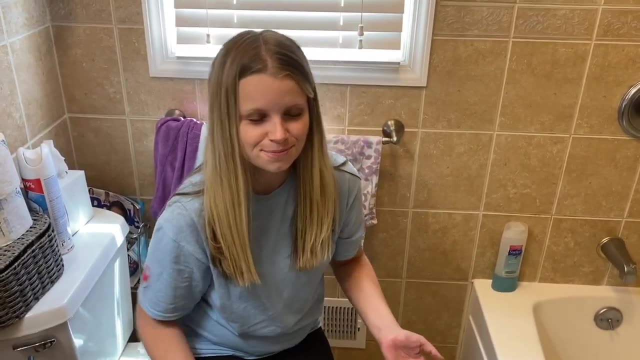 Sit back down And, with your hands or if someone is holding the paper, lift And that's going to start your body. After you do your foot, it's important to use soap and water to get the paint off the bottom of your foot. 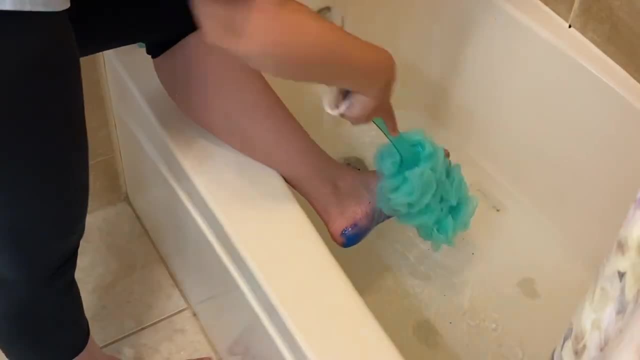 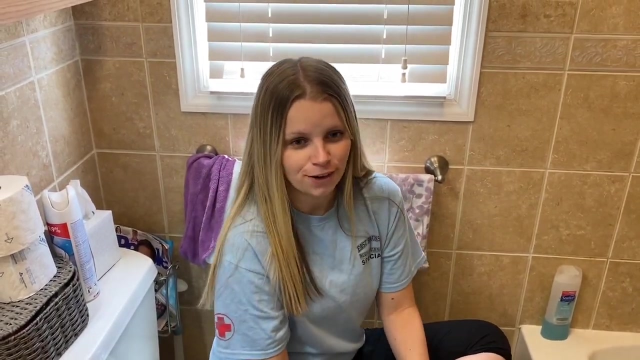 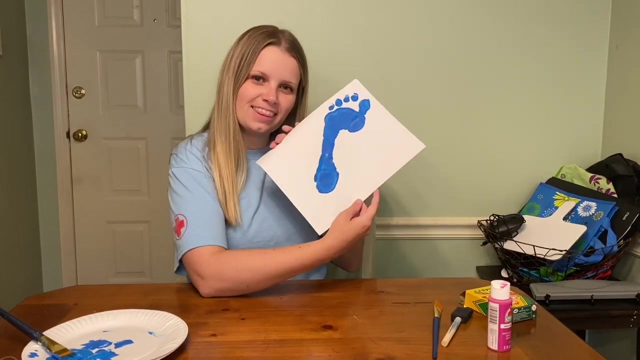 It will come right off. After rinsing off the paint from your foot, make sure you grab that towel and dry your foot completely. So we just finished the body of our superhero and it should look a little bit like this. So I'm going to go in and add a little bit more detail to the body of my superhero to make it look a little bit more even. 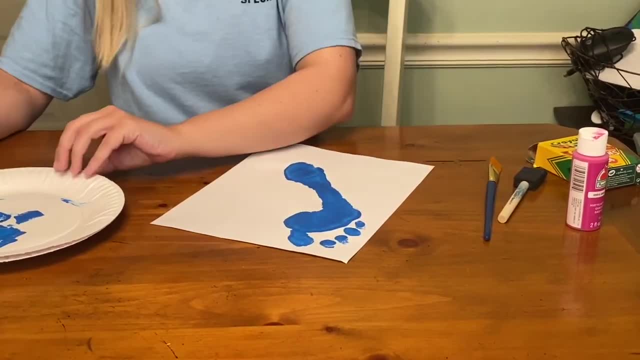 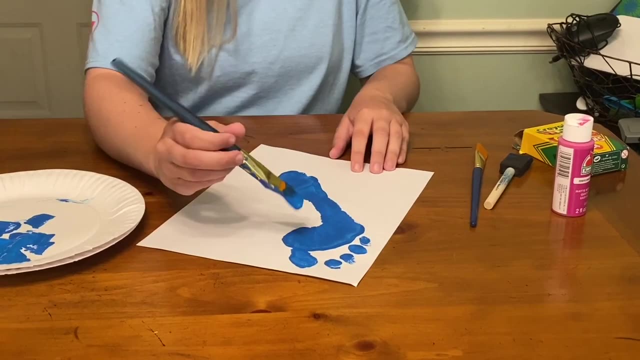 This is totally optional, which means you do not have to, but I'll show you how I would do it. So I'm going to make a little line that connects from here to here. With your paintbrush we're going to go in. 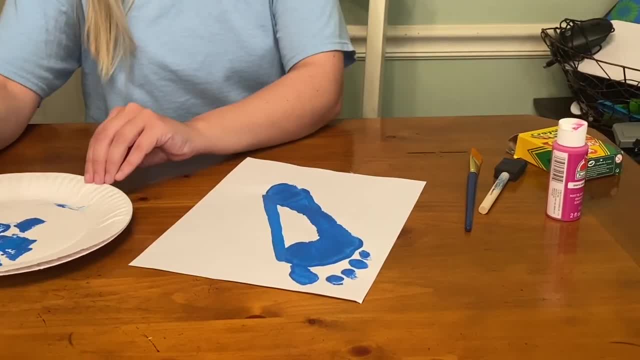 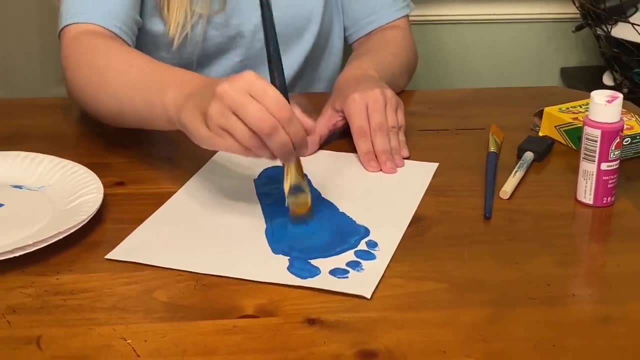 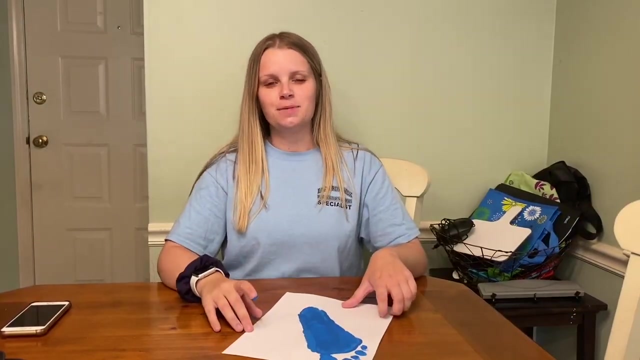 Connect to that line And now we're going to fill it in with paint, with our paintbrush, And that's going to finish the body of our superhero. So the next step in our body is to make the superhero's arms that are going to stick out in front of him or her. 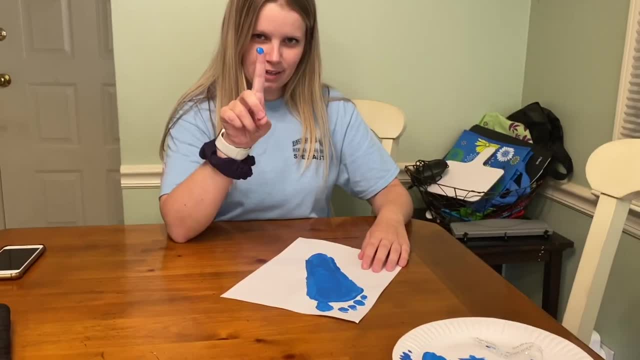 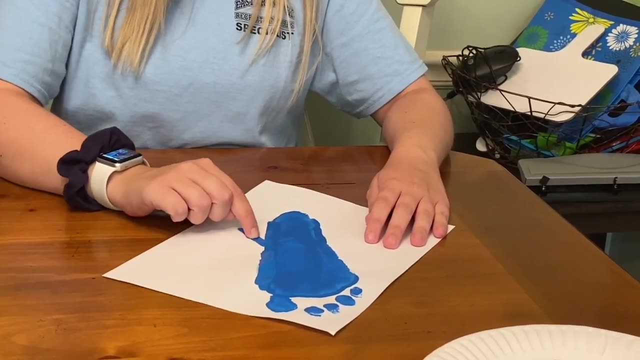 So I'm going to take a little bit of paint on my fingertip and just make a little line sticking out like that. And that's it, Thank you, And that's going to make their arms. So the next step is going to be to paint our hand with our cape color. 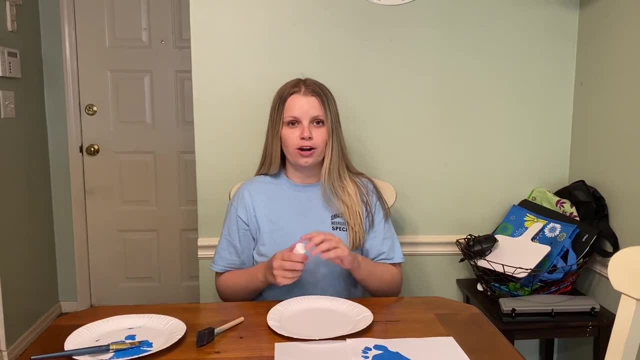 I chose pink, but you can choose whatever color you want. This is going to go on our hand, which is going to make the cape on the back of the superhero, So you can do this right on your hand. You could do it on a plate. 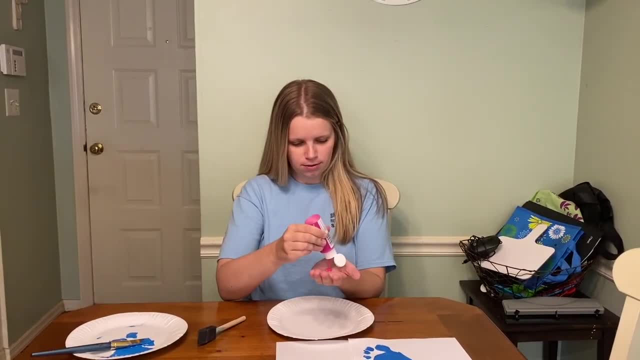 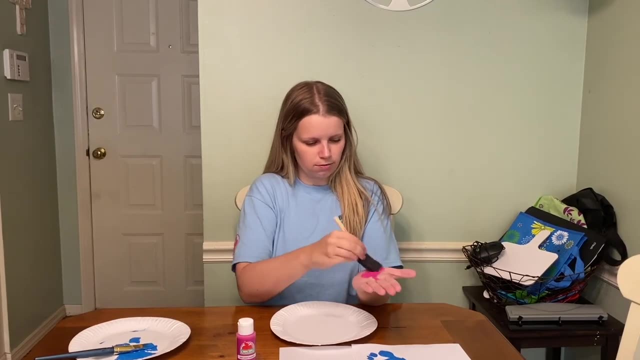 Whatever works best for you. I'm going to put it right on my hand. This doesn't cause as much paint and mess as it does when it's on your foot, And I'm going to take my foam brush. I'm just going to spread it around my hand. 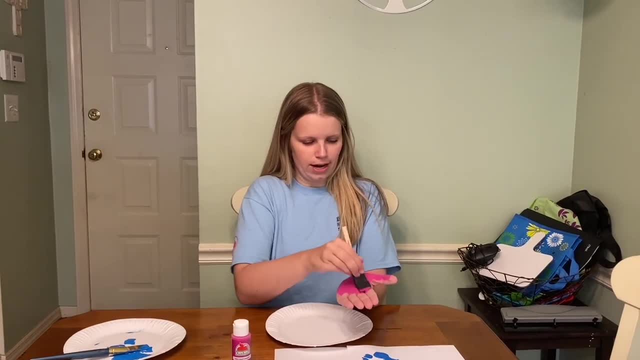 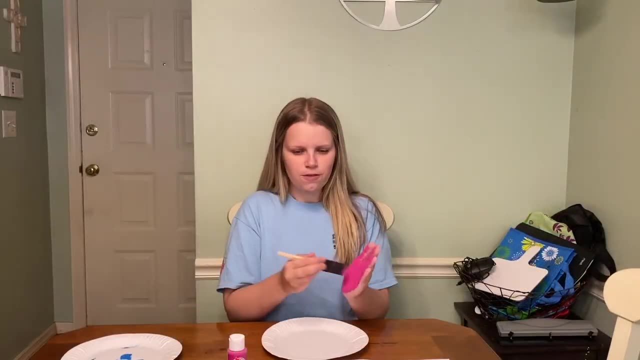 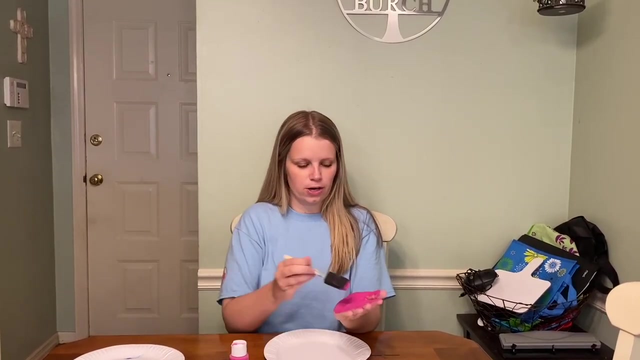 To make the full cape effect when we put it on our paper, And it should look something like that. If you want to, you can add a second coat, So I'm going to add a little more paint to my hand And spread it around again. 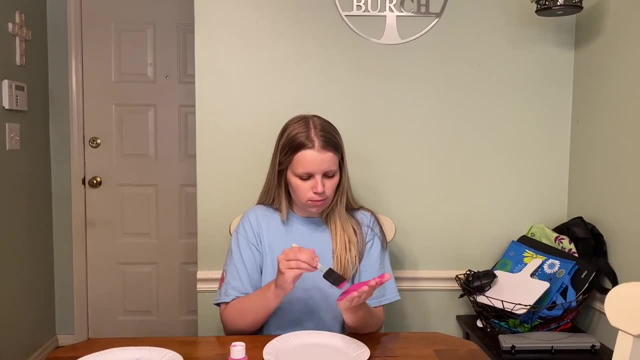 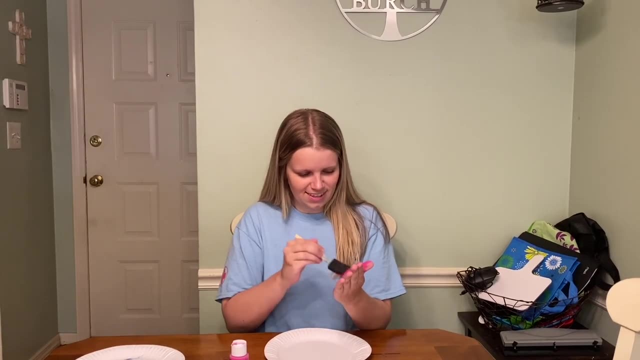 Like we did with the foot. the second coat can make it look a little bit more thicker and a little more bold, And if you need to go in with more detail at the end, that's okay too. So it should look like that. 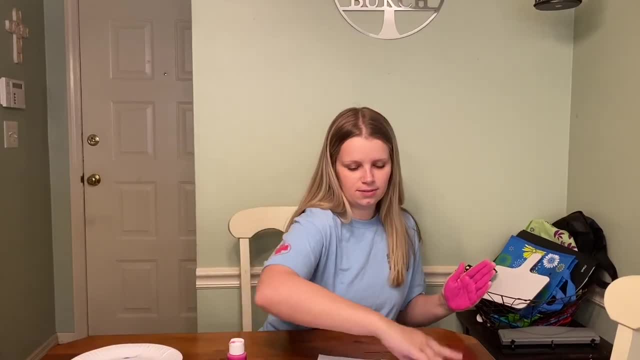 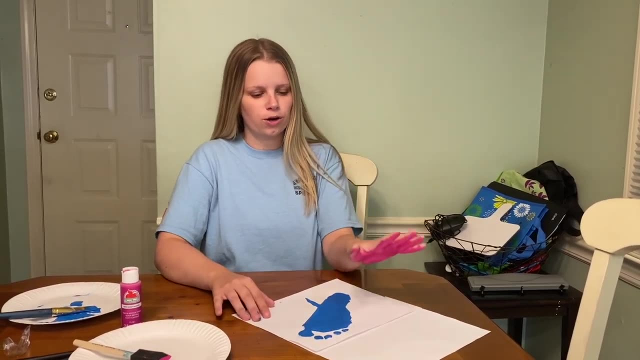 It's covered in paint, So it's time to put on. So it's time to make our cape. Our hand is covered in paint in the color that you want to be your cape, So we are going to match our pinky toe to our thumb. 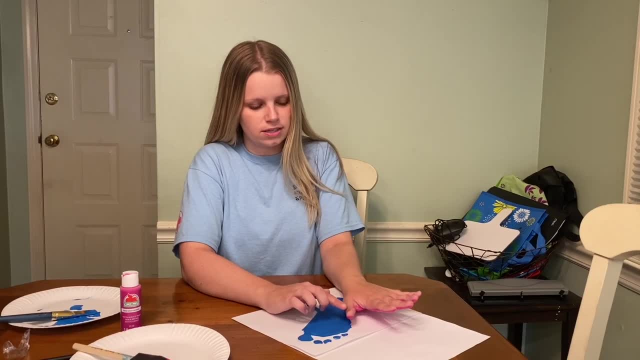 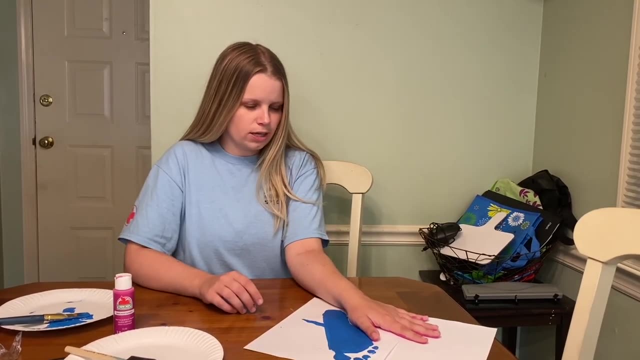 So they are going to be friends here And you're going to leave your thumb on the side of the foot. I added two pieces of paper because I have a big hand, But if you have smaller hands, normally it fits on one piece of paper. 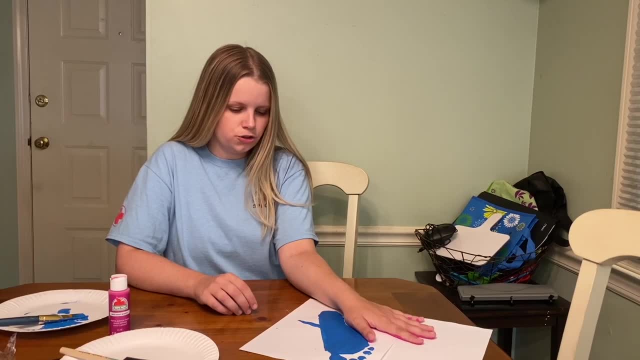 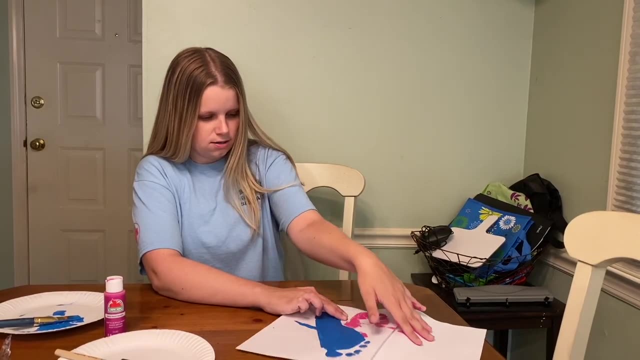 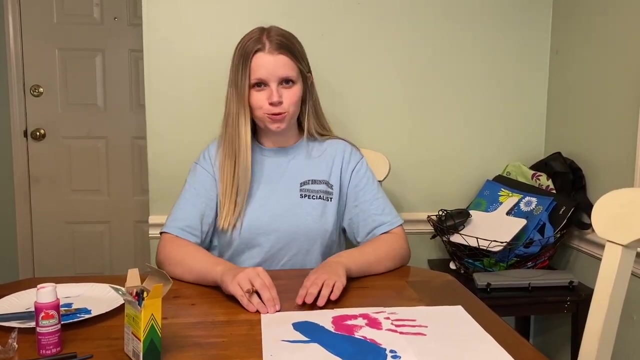 Leave that for five seconds. One, two, three, four, five. Hold the paper for balance And lift your hand. It should look something like that. So the next step is going to be to draw the head and the hands of our superhero. 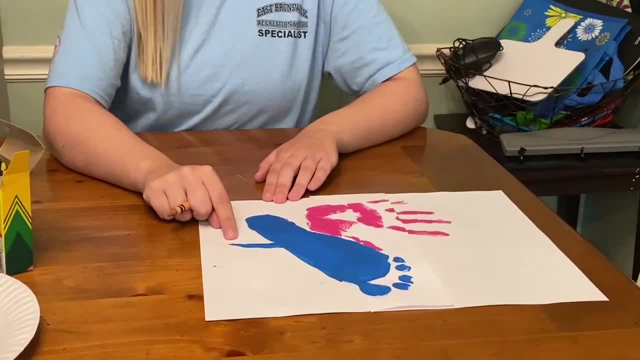 So we're going to go right to this line that we drew earlier And we're going to draw their hands. You can draw fingers or you can draw a fist. I'm going to draw a fist because it looks a little more superhero-like. 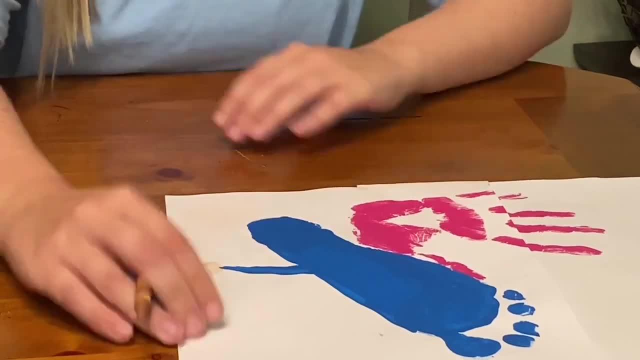 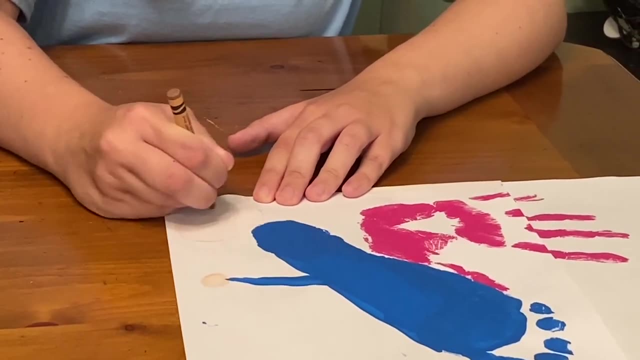 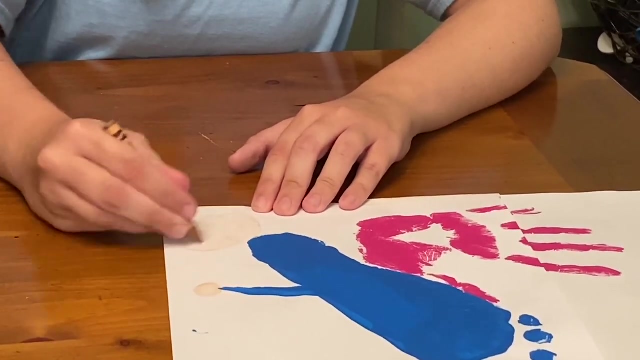 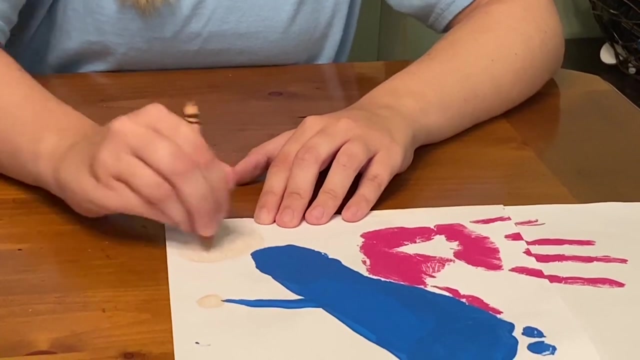 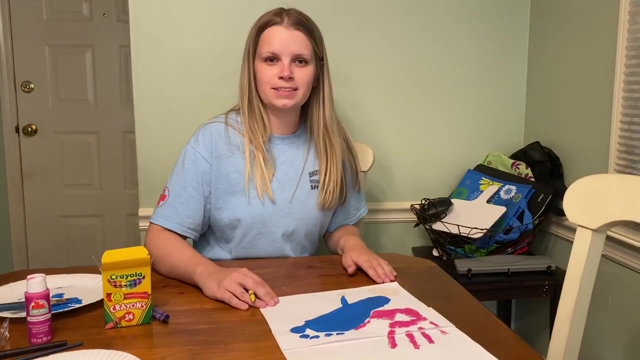 Then we're going to go to the head, Outline that head. You can do it a couple times if you want to make it dark And color it in, And it should look something like that. So the next step is going to be to add details to our superhero.